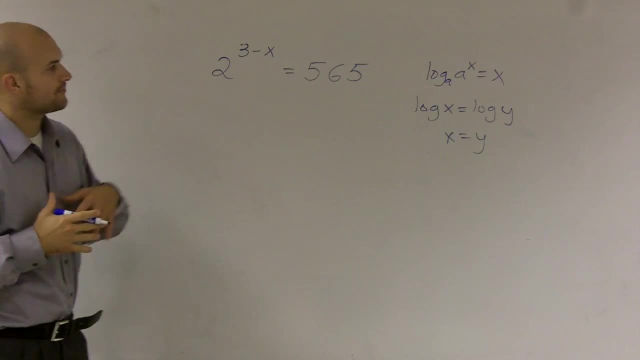 So you're going to have to equal each other. So if I look at this, I need to get this off the bottom. So whenever you have an exponential function, there's a couple ways you guys can look at this. Whenever you have an exponential, you can also look into transferring it to logarithmic form. Or you can also look into it as saying: how can I get rid of this by taking the log of both sides. So if I take the log of both sides, I need to choose my base. 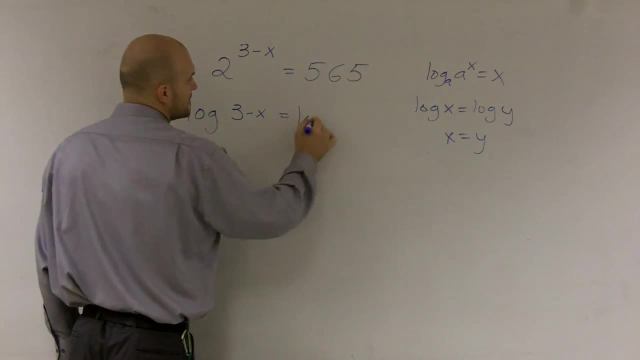 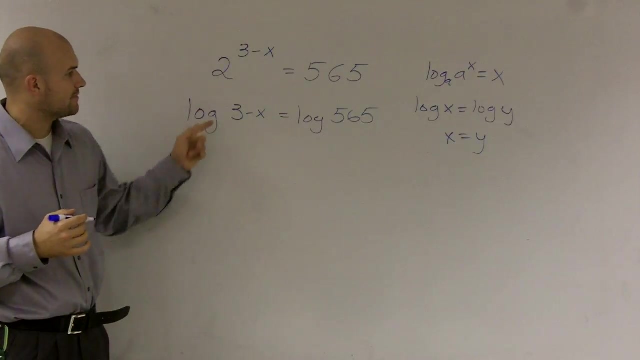 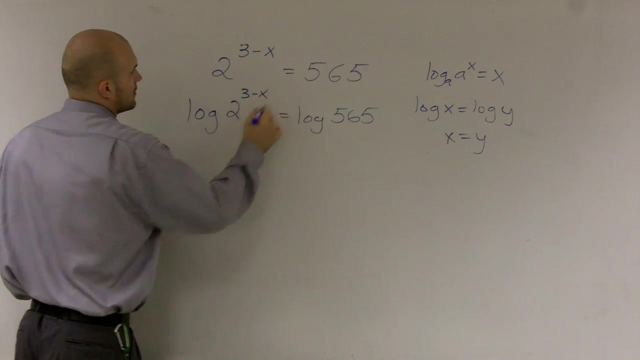 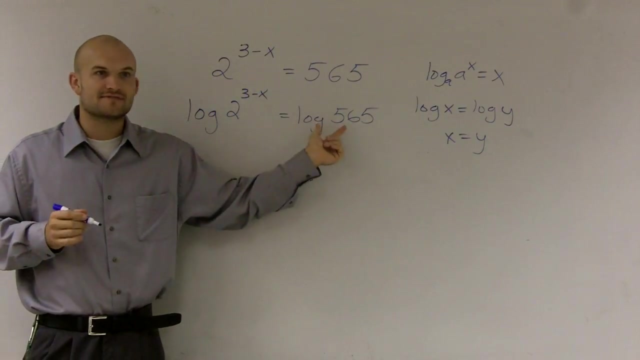 That I'm going to take the log of, And obviously what I want to do is, since I have this variable here, I want to get rid of log base 2.. I need to get rid of this 2. Why? Because that 3 minus x is an exponent. I need to get rid of this side. So you wouldn't want to make the base 565.. You'd want to make the base 2.. So then you can get rid of this and just 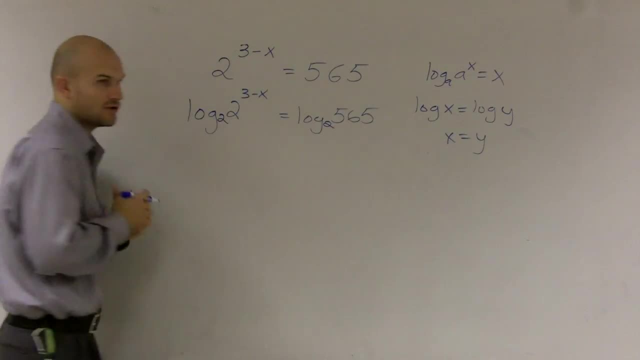 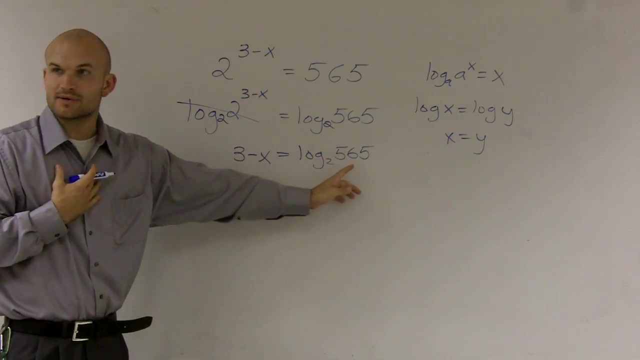 leave your exponent, So I'm going to have to take the log of base 2 of both sides. Then what happens is that cancels out to give me 1.. I'm just left with my exponent, which is: 3 minus x equals log base 2 of 565.. Now I can just do solving my equations. I know that's a crazy number, right, But really all it says is: 2 raised to what number gives you 565, right, Just? you don't need to worry about figuring out right now. 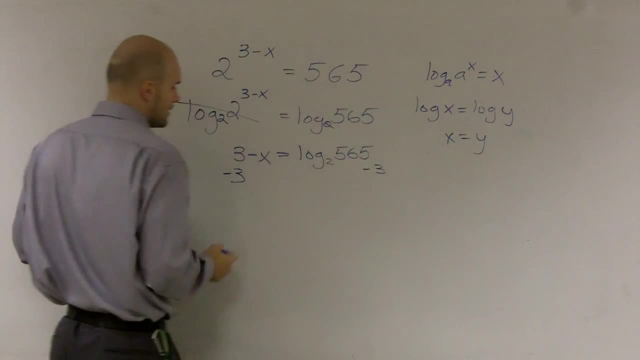 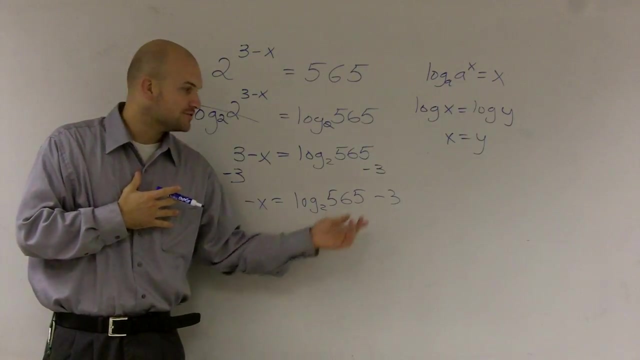 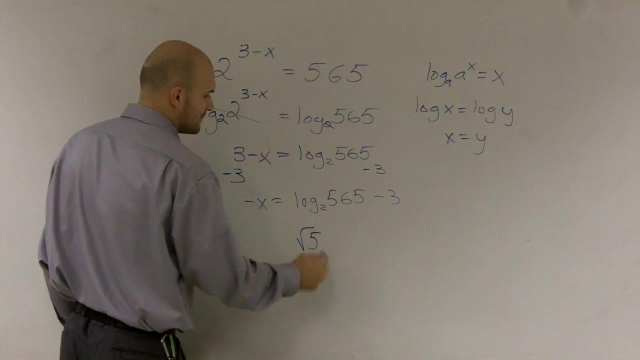 Just subtract your 3.. Alright, so you have negative x equals log base 2 of 565 minus 3.. Please, ladies and gentlemen, please remember that logarithm is a function. Okay, Do not subtract your 3 from times 565.. Because I know you guys don't do this. Or, hopefully, If I say negative 5 minus 3, you guys should understand that you can't make that 565..